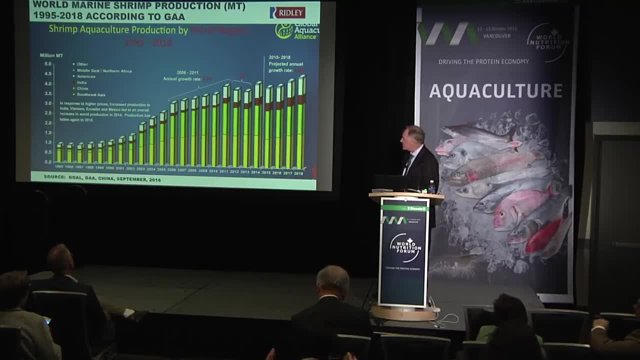 as the production from world shrimp farming increases year on year. A couple of blips here and there, especially over the last couple of years, but the prediction is that it's moving forward at about 4% per year for the next few years. I think that this looks great on paper. 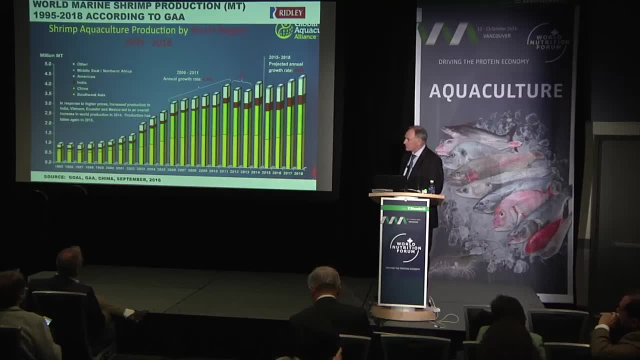 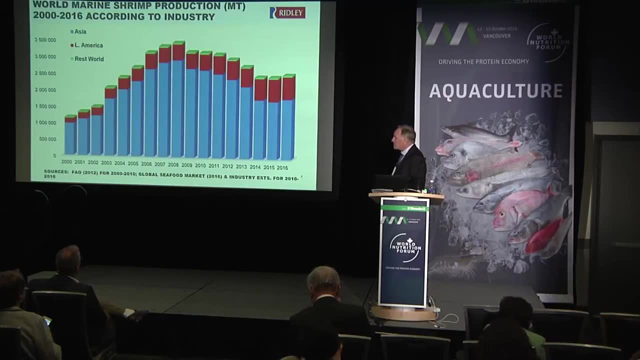 but actually bears very little resemblance to what's the real truth, And I think that looks a bit more like this And you can see here this is actually information using FAO figures up to 2012,. but then they get a bit hairy. There was a global seafood market. 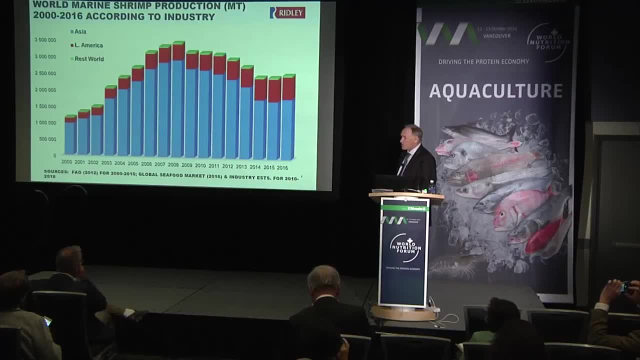 conference in 2016 and industry estimates were incorporated in that, and I think this gives a much more realistic picture of what's really happening. and you can see, since about 2009, there's actually been a decline in production. the reason for the discrepancy between these two figures is that the data 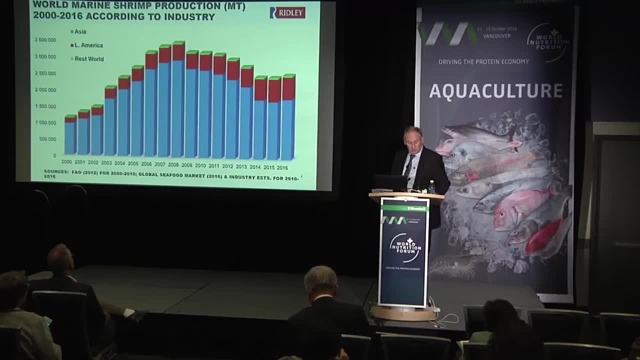 provided to FAO, which forms the basis of the global aquaculture estimates, is overstated, particularly by the Chinese and the Vietnamese and to some extent the Indonesians, and that skews the whole scenario. you can see. still, most of it is produced in Asia, from a peak of about 84 percent of shrimp production now down to 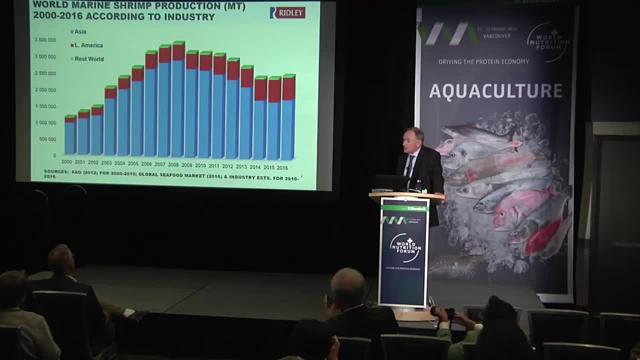 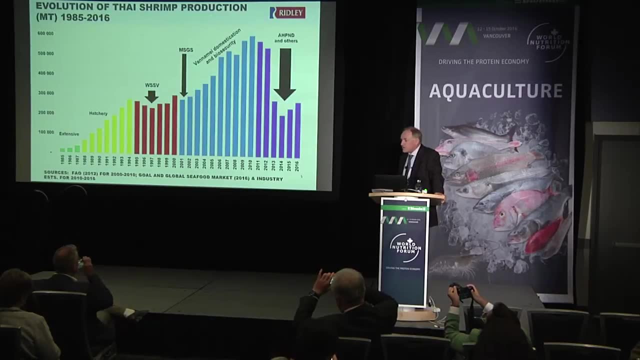 about 77 percent, with South America taking a larger share as it's less affected by these newer diseases, particularly EMS. having a look into the individual countries, I'm just going to use two examples: Thailand and then Ecuador, which gives a real indication of how diseases have impact the 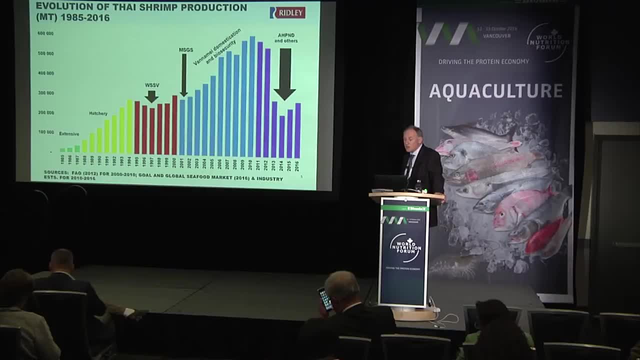 structure and the development of these individual countries. aquaculture, prawn farming industry. you can see, at the beginning, back in 85, it was a very extensive system. we're using wild post larvae. then the hatchery was invented and brought into production through the late 1980s, early 1990s. then along comes. 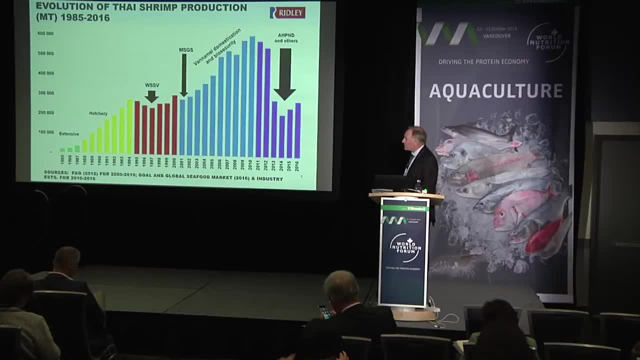 white spot disease. this is all for monad on in these early days. white spot disease came in the middle 90s put a big dent in that industry. it started to show some kinds of recovery again with monad on, but then monad on slow-go syndrome came in and really forced the conversion in Thailand and 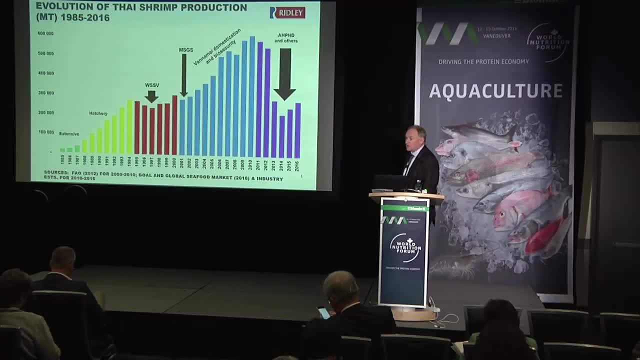 the rest of Asia from monad on into vanamite. so this was using imported SPF stocks from the Latin American or North American brood stock industry and the combination of these two factors is a very significant improvement. in the combination of the introduction of vanamite and the SPF stocks, the 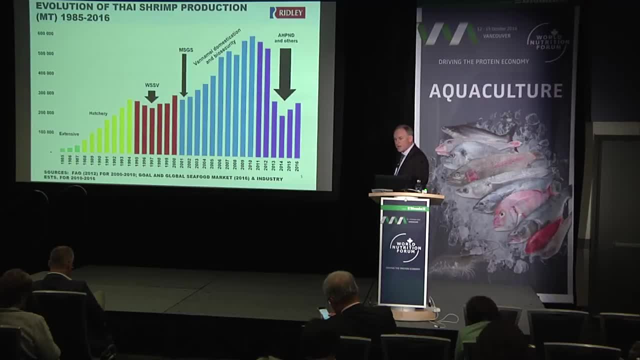 domestication. that and selection of faster growing animals and biosecurity measures that were employed in these smaller Asian farms led to this explosion in the culture of vanamite in Thailand, which led up to about six hundred thousand metric ton per year production. then along came a HP and D or 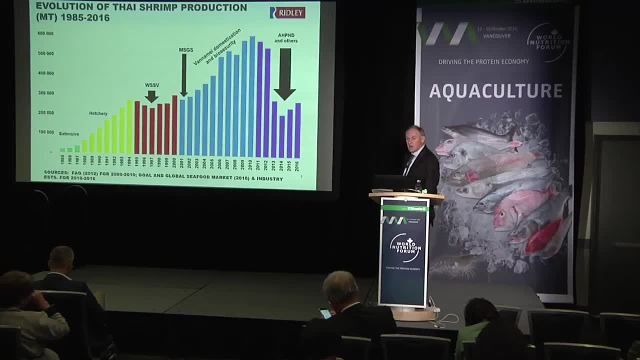 EMS and you can see what kind of effect that's had, that it's halved at the production or more, and continues to affect the Thai production right now, and this is a very similar situation to what's happened in the other countries that EMS has affected, including China, Vietnam, Malaysia, by 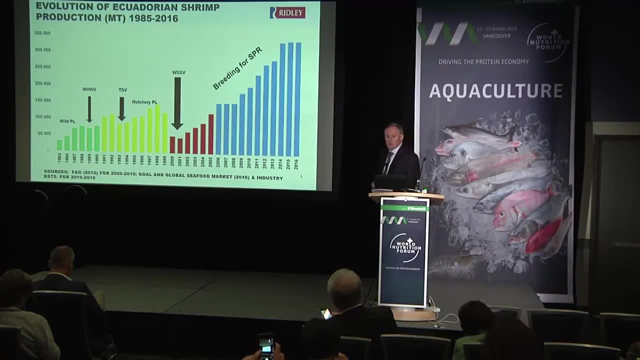 contrast, if you look at the evolution of the shrimp culture industry in Ecuador, again, we can see that there's been periodic outbreaks of disease that have come and affected the production of vanamite and these stocks have been the production significantly. This first started with IHHN back in the late 1980s. 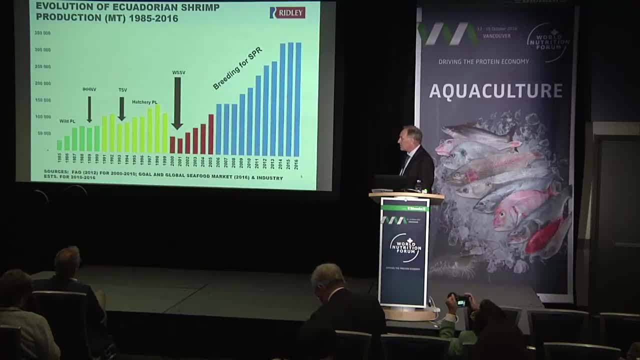 Tower came along in 92, 93, had a moderate effect for a short time. Hatcheries built up. This is all for vanamai. Then in 1999, along came white spot and put a serious dent in the industry. 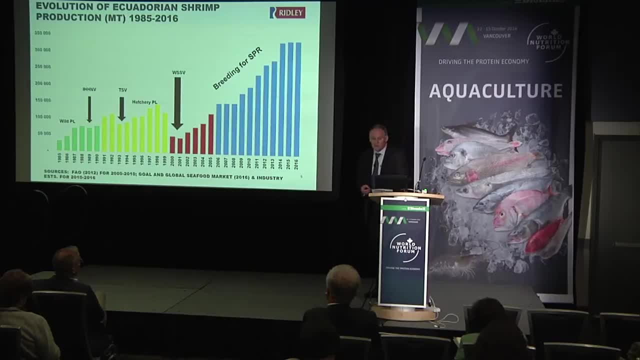 That persuaded people to start looking at specific pathogen-resistant strains of animals that were resistant to white spot. That has continued today. They are continuing to increase their production, so that their production is now higher than that of Thailand. They haven't yet experienced EHP. If that does happen, I would expect a similar scenario to what's going on in Thailand and the rest of Asia. Right now, Ecuador is doing very nicely In terms of the shrimp diseases. traditionally, the most important ones were the viral diseases. They've developed over time, so there's now more than 20 different viruses affecting Paneid shrimp. 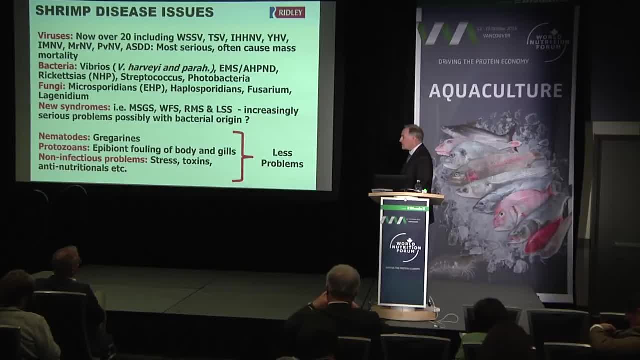 These are often the most serious and cause mass mortality in a very short period of time. More recently, the emergence of bacterial-derived diseases, like with the vibrios that are causing EMS, and now with fungal problems like the EHP, micro-spiridians and new syndromes that we still 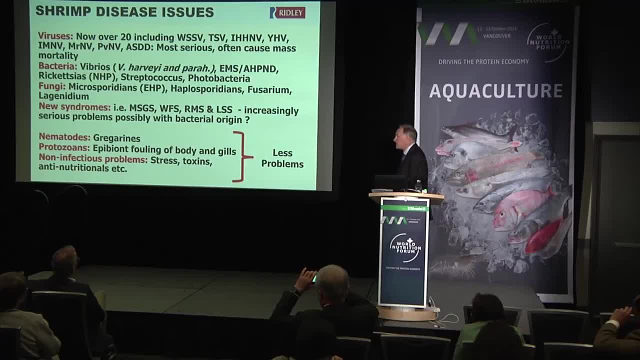 really don't know what they are. These are having a very serious effect on the health of the shrimp. These are having more effect even than the viruses did. Then there are less serious problems like nematodes and protozoans and other non-infectious problems. I mentioned about this loss due to disease. There's been a lot of work done prior to the arrival of EMS looking at how much the industry has suffered due to disease. There was various estimates: up to 40% of total production, 15 billion dollars, 80% of which was from Asia. 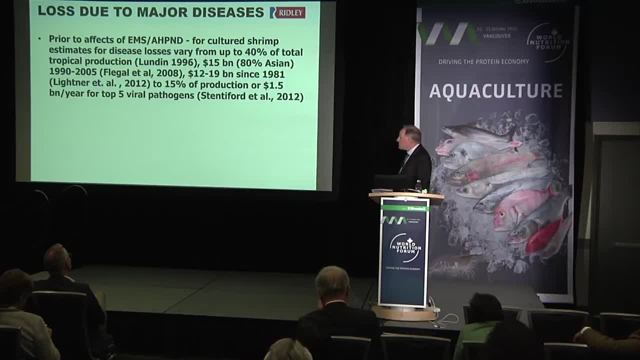 19 billion since 1981, or 15% of the production, or 1.5 billion per year for the top five viral pathogens. This was all prior to EMS. As a result of this, the World Bank recommended that the industry should be. 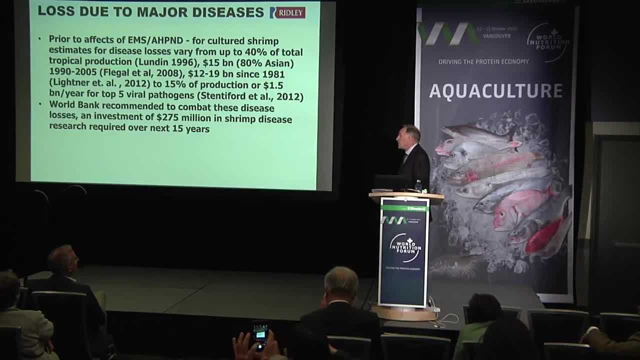 investing at least $275 million over the next 15 years to combat these viral problems. At that time, viruses were accounting for about 60% of the world's population, of the disease losses in shrimp, aquaculture and bacteria about 20. but as 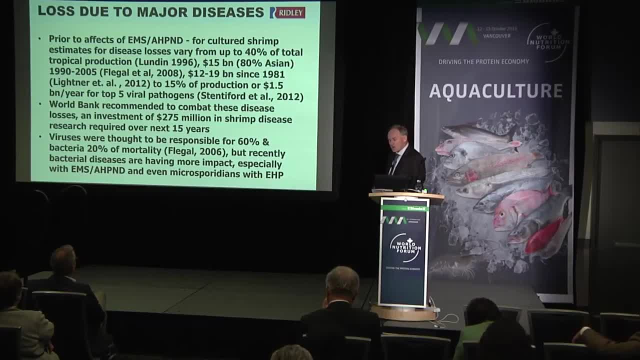 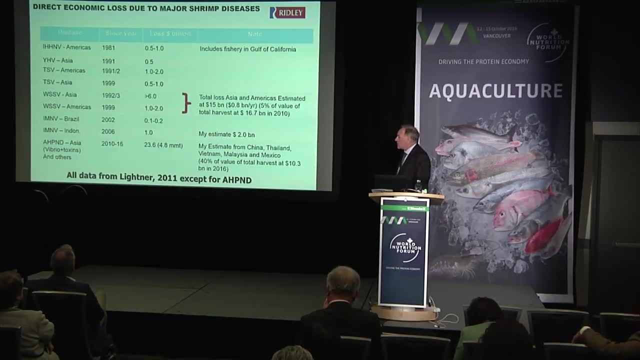 I mentioned. with the recent introduction of EMS or HP and D into the scenario, that is no longer the case. this information is largely from lightness paper in 2011, which kind of goes through the history of the losses caused over time due to all these various viruses. the most significant one was white spot. 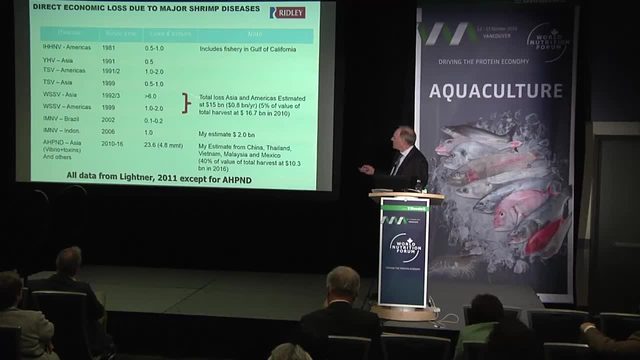 both in Asia and the Americas, which was resulting in about 15 billion dollars of loss between 92 and 2011. that's about 5% of the value of the total harvest then we had- I am in V in Brazil, and then Indonesia, and now we have a HP and D not. alone, but in concert with other disease issues that are occurring, and the estimate that I've derived from this is that we've lost about for 40% of the total value of the harvest, which amounts to some 23.6 billion, with a B dollars of about 4.8 million metric tons. that's just between 2010 and 2016. 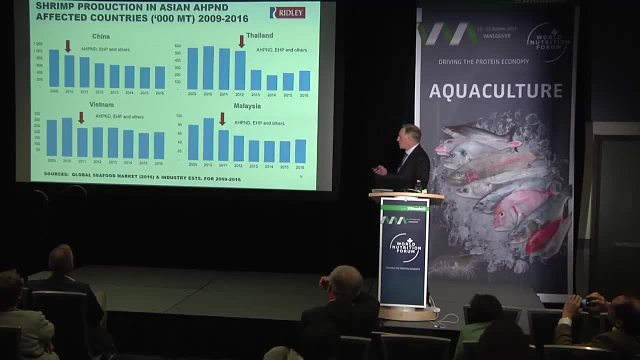 how is that played out country by country? if you look at China, the official statistics from China will tell you they're producing over a million up to a million and a half metric ton per year. that's absolutely not true. the more lightness paper is the one that is the most likely to be the cause of the loss. 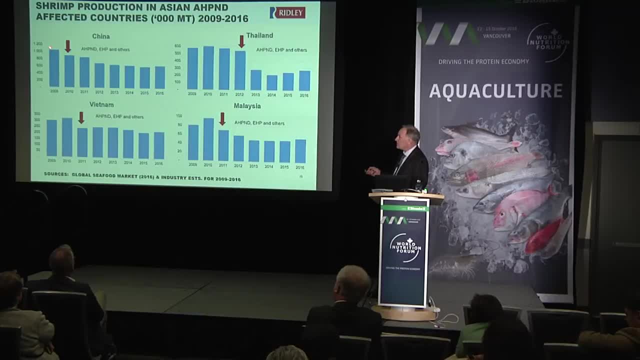 estimate is somewhere where they've declined from about just over a million down to about six hundred thousand ton. this was from the global seafood market report and this is a direct result of a HP and d HP and a few other diseases thrown in for good measure. Thailand, as you've seen, gone from about six hundred. 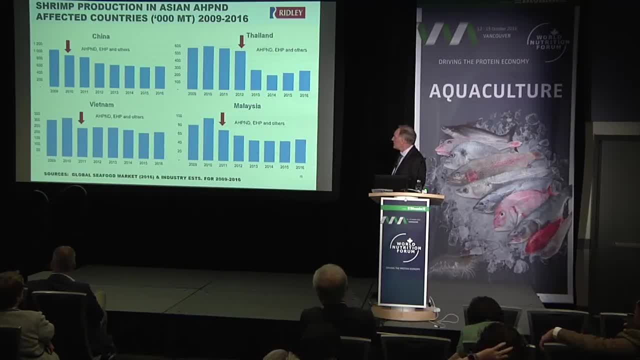 thousand tonnes, down to 200 to three hundred thousand tonnes today and really not making a spectacular recovery as yet. Vietnam, similar scenario: they're down about 200 to 250 thousand. and Malaysia, since the introduction of HP&D, similar cause, where they've gone from a hundred down to about 50,000 metric tonne. EHP also went. 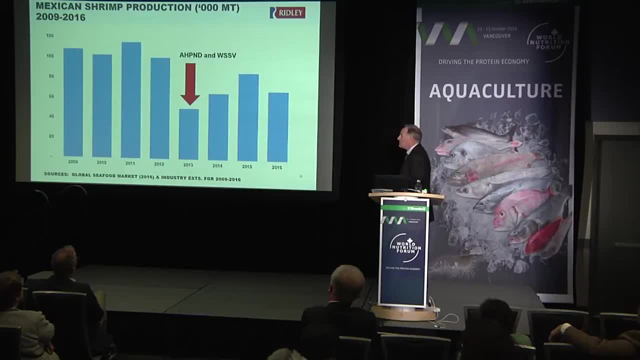 over to Latin America starting in 2013 and it entered Mexico and we had this very similar scenario where productions gone from about a hundred thousand tonne down to 50. they made some improvement through the selection of disease resistant stocks, but it's quite variable. they're still struggling, if you. 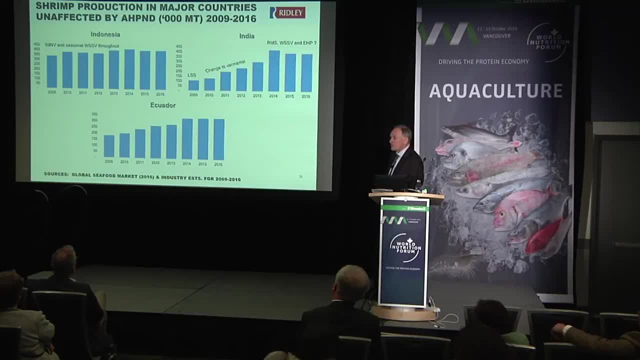 look at that, in contrast to the countries, the few countries- that are not suffering from HP&D right now, like Indonesia- sorry, we still have problems with IHN, IMNV and white spot, but the production has been maintained fairly stable- India has increased its production quite a lot from their. 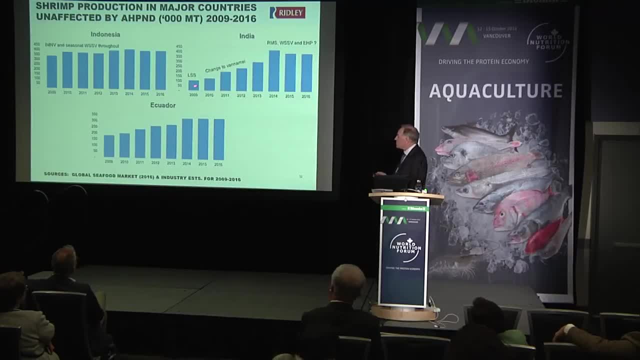 hundred thousand tons producing purely monodon. they changed belatedly to vanamite and the production has gone up quite considerably. but now they're suffering from other problems like run, like running mortality syndrome, white spot periodically and also EHP. so their production is also leveled off and then, as I showed you before, Ecuador continues. 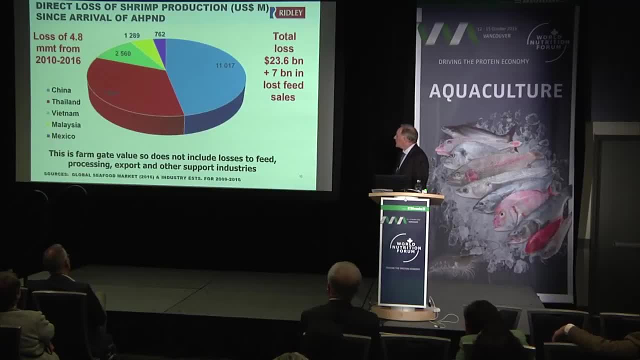 to improve in the absence of EMS. so that figure breaks down something like this to about twenty three point six billion dollars. that's just in lost production, that is, shrimp that have either died or have not been produced as a result of EMS and other diseases being in the environment. 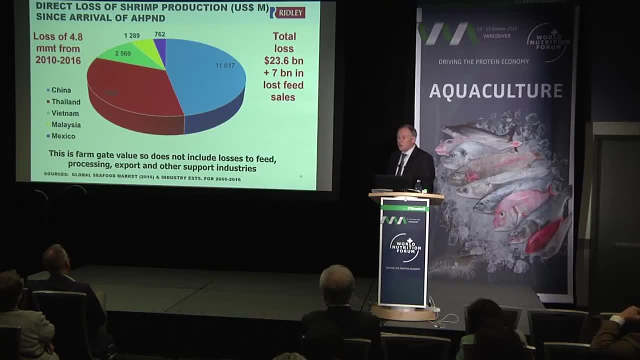 right now. you can add to this at least seven billion in lost feed sales, and then there are also losses in terms of unemployment, in terms of the processing and marketing and distribution of the product that is not being produced right now. so you can see, a lot of this is originating from losses in China, and 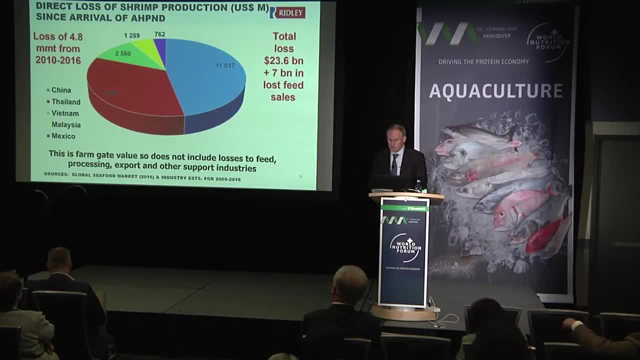 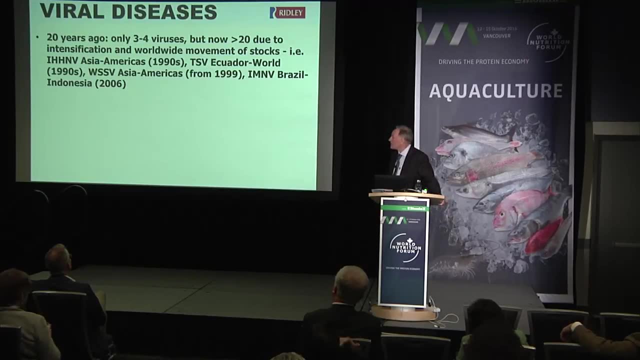 Thailand, six ten, Vietnam, Malaysia and Mexico. so, in terms of viral diseases, as I said, twenty years ago there was very few of these around, only three or four. now there's over twenty, and a lot of this has been derived from the globalization of shrimp farming and the introduction of vanamite from Latin America into the rest of the. 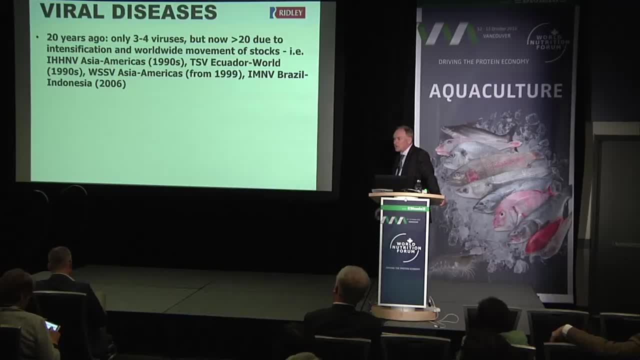 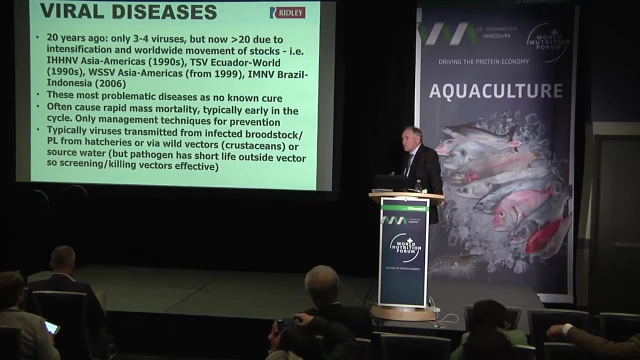 world and it's brought with it, in many cases, some of the diseases that were affecting it from its home nation. these are the most. these have been the most problematic and there's no known cure for any of them. they often cause rapid mortality and they're often transferred from infected. 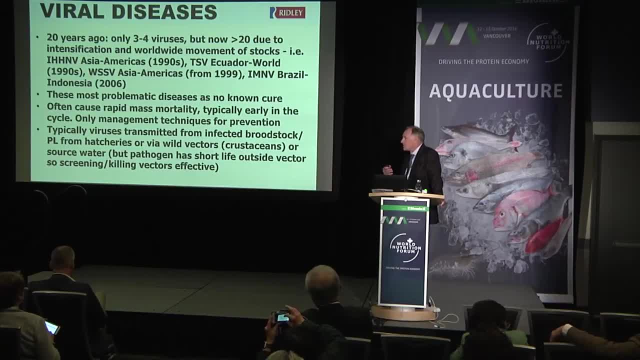 broodstock that are often taken from the ponds and transmitted through the hatchery, through the PL, into new sites. they rely on transmission through wild vectors, typically crustaceans, or through water, but a lot of them have a very short life outside of these crustacean host organisms. so if you can, 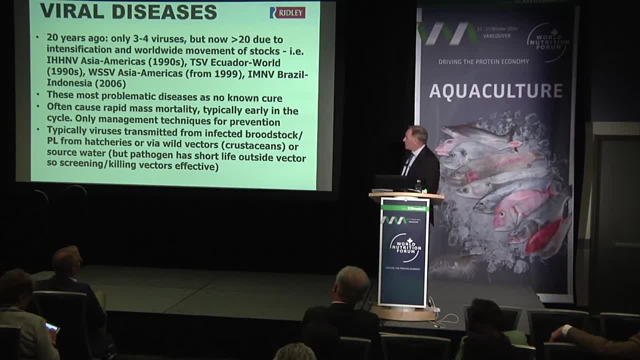 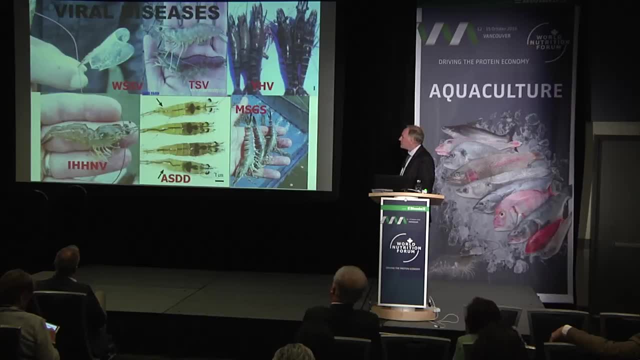 get rid of those, those vectors, then you can help to control the transmission of the disease. this is just some pictures of the various viral problems that we've seen over the years, with white spot which continues tower not such an issue anymore. also, yellowhead IHHMV is continues to be a problem causing. runting and slow growth. this is a new one called abdominal segment deformity disease, which is also thought to be caused by a virus now, and monodon slow growth syndrome, which caused that transfer from monodon to vanomai in most of Asia. then there are the white-bodied shrimp viruses, which includes the IHMV. 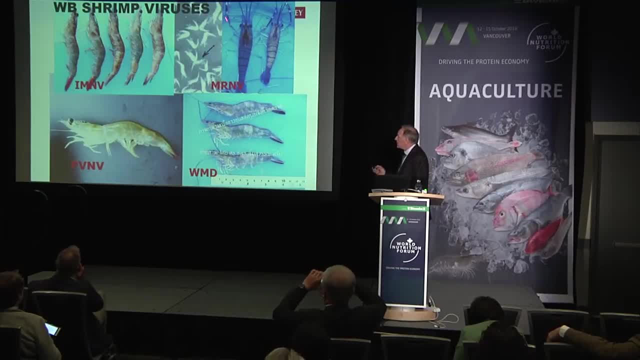 originating in Brazil and moving over to Indonesia. macrobrachium rosenbergii notavirus, which looks very similar to this, originally happened in macrobrachium and then was transferred into vanomai Paneus vanomai notavirus, which is another very similar virus, which is a very similar type of virus, which is 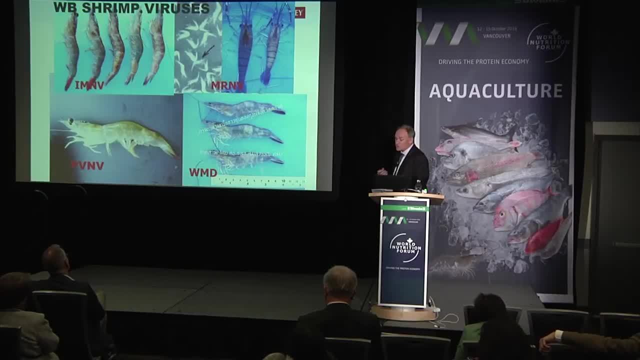 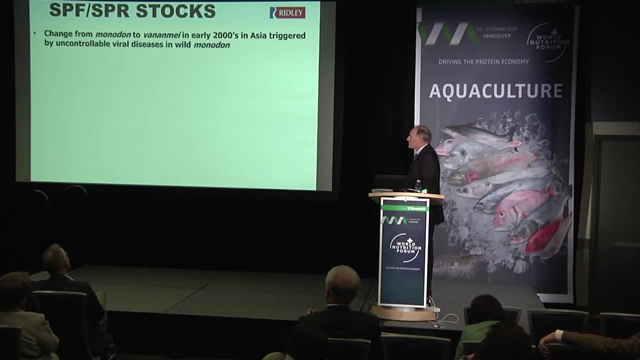 similar looking disease. and then there's a white muscle disease which, as far as we know, is not caused by a virus but looks very similar to these others. this I feel ought to kind of mention about the SPF and SPR. this introduction of this domesticated, selected animal from Latin America into Asia really spurred 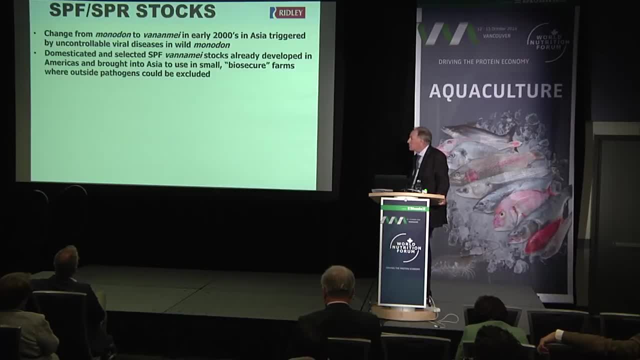 that change from monodon and that massive increase in production we saw in Asia. this was because he already had the availability of these SPF stocks, which had already been domesticated and in some, in some instances, selected for improved disease resistance and faster growth. but the SPF paradigm didn't really work in these. 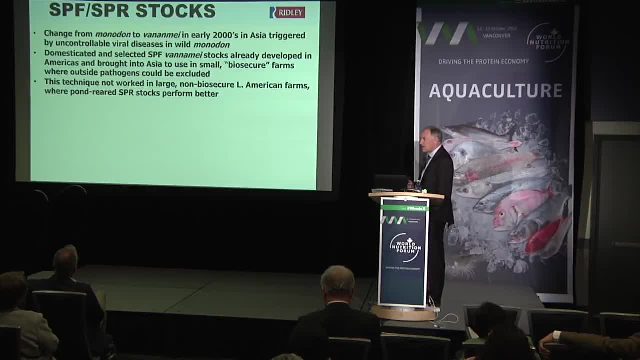 large, extensive Latin American farms. they instead had to go for specific pathogen resistant animals that were selected in the farm itself. when you stopped SPF stocks they went into the ponds and the farms free of disease, but they didn't stay that way very long so it didn't work out for them. there are some spf sbr stocks for taura, for white spot, for imnv now in. 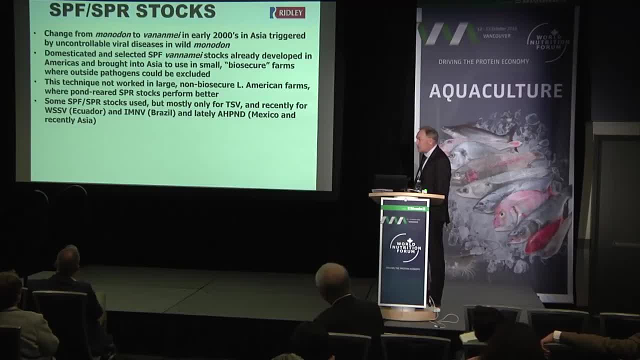 brazil, and lately there's been some developed for ahp india as well, both in mexico and recently in asia. in asia they originally started bringing in a lot of animals- the spf animals from hawaii- but over time that number diminished and diminished as they started producing these stocks. 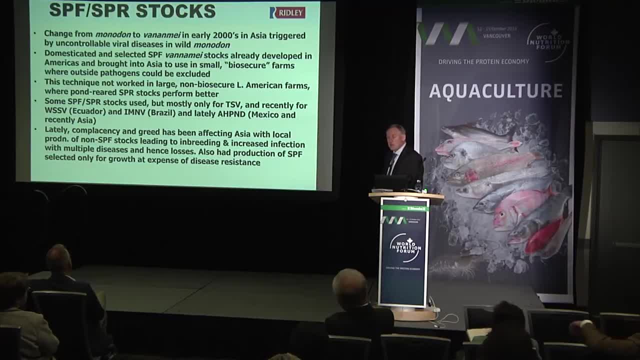 themselves. but they didn't tend to maintain that spf status. they started selecting animals- good performing animals from the pond which were infected with multiple diseases and that has caused a lot of problem for the asian industry. now they also have some spf selected animal, but they did that selection based purely on growth, not on disease resistance. 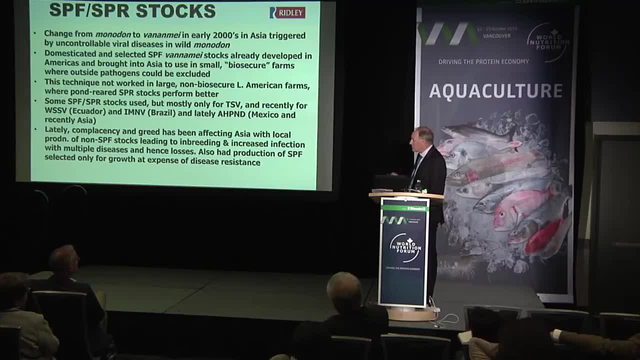 and that has come to back to bite them with the introduction of ahp and d. so we really need to look much closer into the development of these spf and spr stocks to maintain our biosecurity and the ability of the animals to thrive in the presence of these multiple diseases. 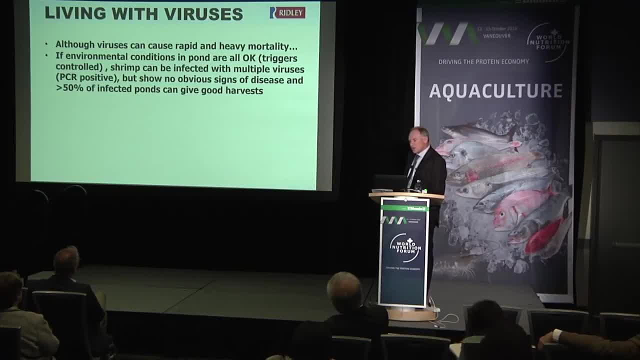 so living with viruses. as long as you keep the conditions in the pond in good condition, the environment certainly is not a good thing for the animals in our local communities. the most important thing is the environmental condition. a lot of occasions the shrimp can be infected with multiple viruses, but if you maintain water quality and dissolved oxygen and nutrition. 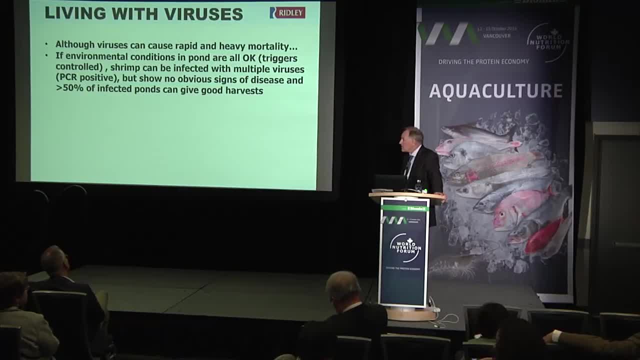 you can get a successful harvest. it's all about the management. there's no treatment for these viruses, but you can still get a good return a lot of the time if you take a lot of care with how you coach your animals. we've had some progress in the development of vaccines. 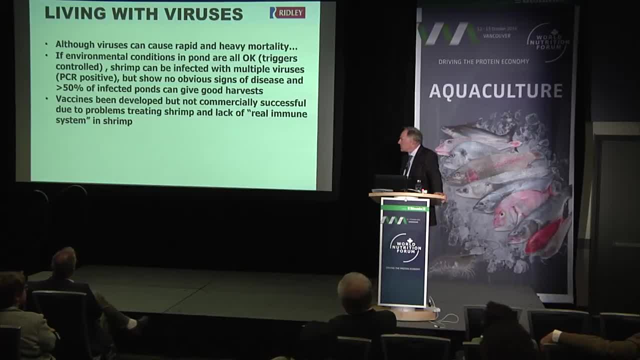 So a true vaccine doesn't really work on shrimp, but there have been some examples, which I'll go into later, which have shown some promise. So, basically, in the absence of real treatments for viruses, we really need to use best management practices to improve the management of our farms, using SPF and SPR animals. 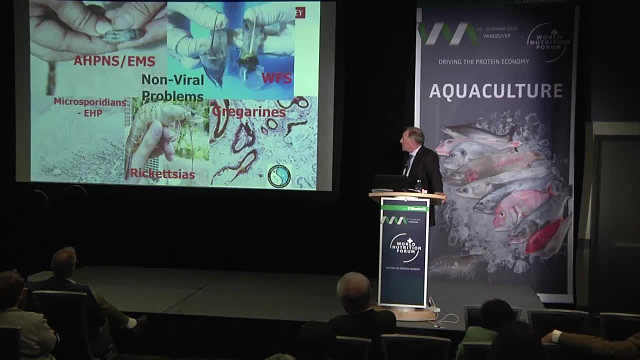 That's about the only way we can survive. Then we move on to the non-viral problems. In principle of these, I'm really going to talk about EMS and white feces syndrome and this EHP caused by microsporidians. 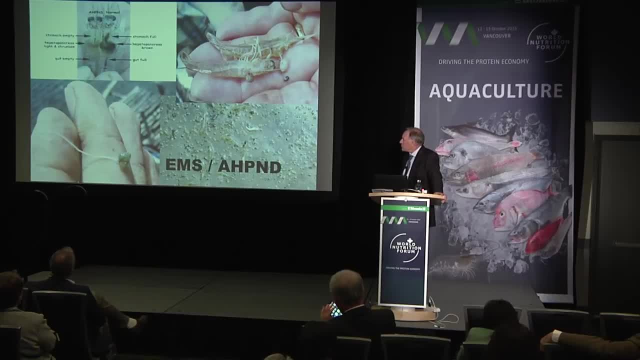 There's a couple of others too. EMS- we all know what that looks like. You get this whitened and shrunken hepatopancreas animals dying very, very early, even before they're a week or two old, in the ponds. So this originated in China In 2009, and affected very young animals within the first month of culture. It went into Vietnam, Malaysia, Thailand, East Malaysia and the Philippines in 2010,, 11, and then 2013,. it got into Mexico. 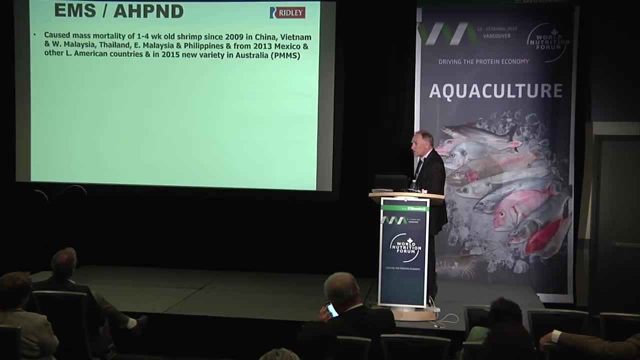 We're not sure how, And from Mexico it's spreading out through other countries in Central America And just last year there was a new variety of this that popped its head up in Australia last year and we're still not really sure. 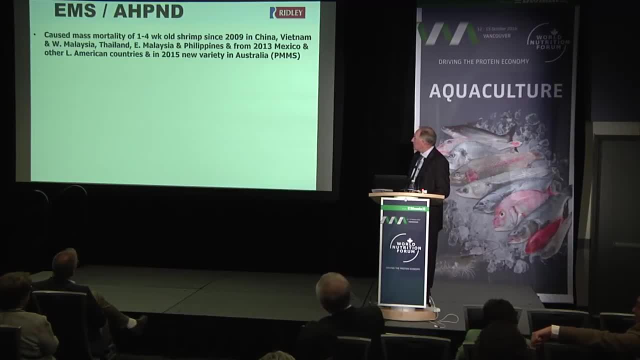 How significant that's going to be. that's in Monodon, but they call it Penaeus Monodon Mortality Syndrome, not AHP and D because there's some differences between the characteristics of the Asian version and the Australian version. We know it affects Monodon and Vanamai. 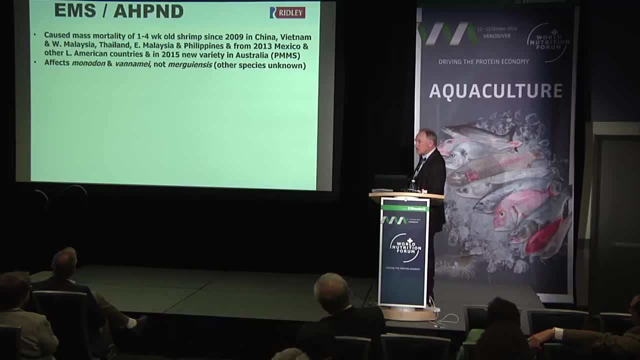 Interestingly, there is a domesticated strain of Merguiensis in Australia and so far it has remained unaffected, even in farms that are infected with the Monodon. So we're not sure how, We're not sure how, We're not sure how. 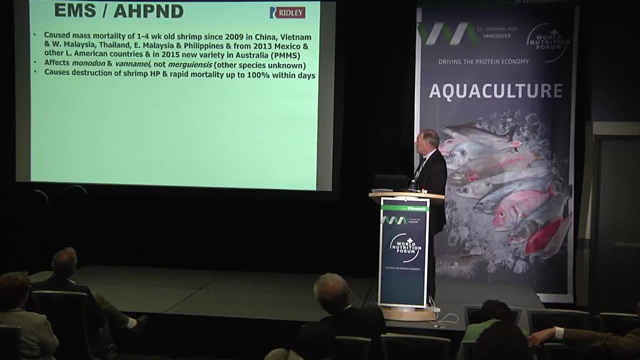 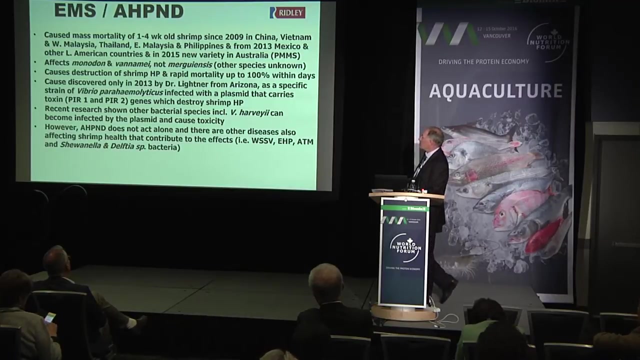 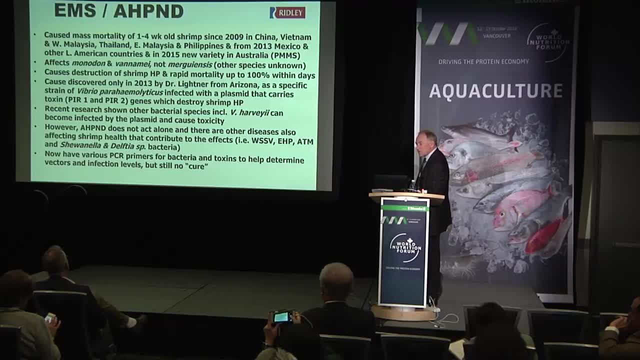 We have various PCR primers to identify both the strain of bacteria and the toxins, so we can look at where it's coming from, how it's being transmitted and how it gets from one farm to another or from the hatchery to the farm. 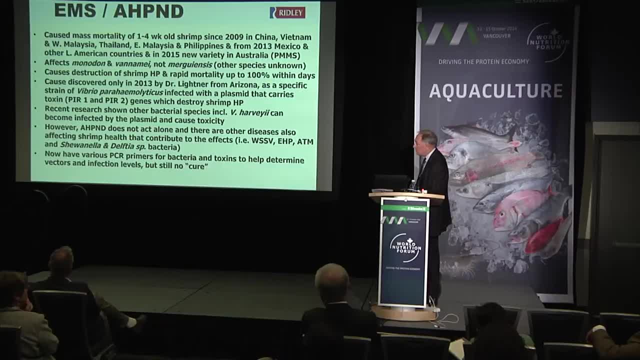 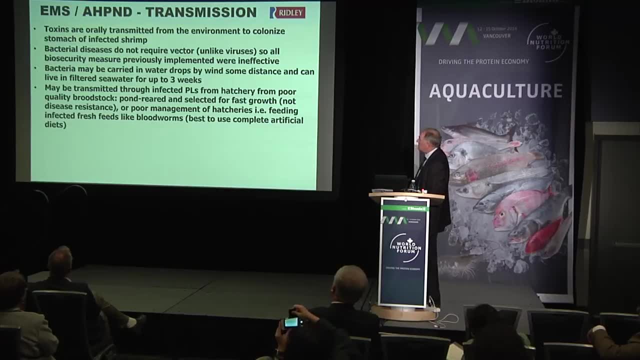 Previously we didn't have that, So now we have a way of finding out what's going on. So the transmission is from the environment to the stomach of the infected shrimp. All the biosecurity measurements that farms adopted to cope with viruses don't work anymore for bacteria. 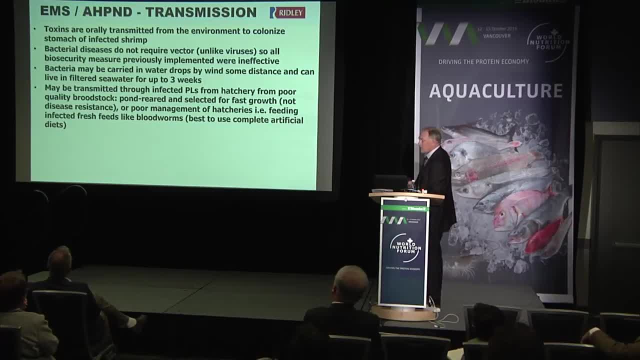 So we've had to rethink the whole system. The bacteria can even be carried in droplets of water and be spread from pond to pond and farm to farm. It's also spread widely through PLs from the hatchery And we don't really still know very much. 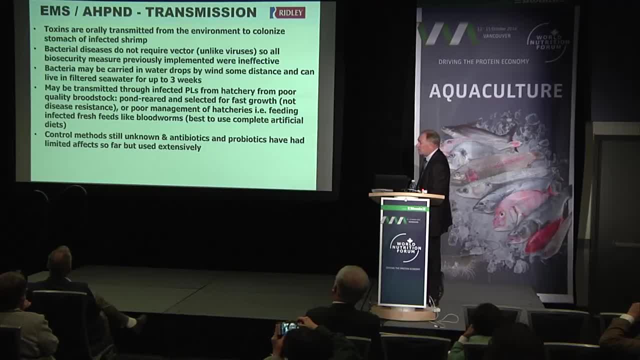 about how to control it. People have been using a lot of antibiotics and a lot of probiotics and they haven't really been very effective. so far, There isn't much risk of importing it in frozen or cooked product, as the bacteria and the plasmid is killed by freezing or cooking. 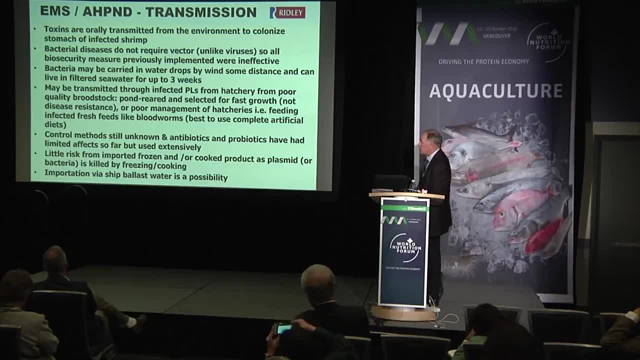 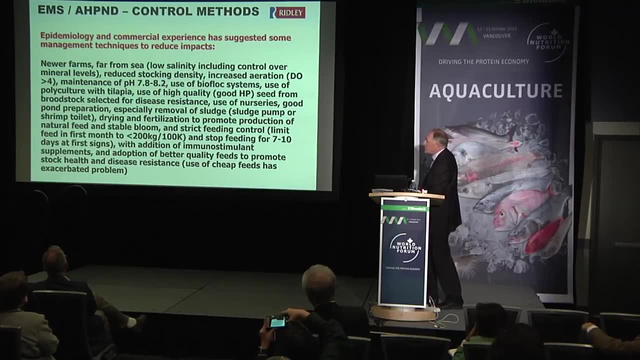 but we're still not sure if it can be brought in by ballast water from ships, but that's a distinct possibility as well. In terms of epidemiology. we've looked at what people do that are successful and we found that newer farms far from the sea. using low salinity have been effective: reducing stocking density, increasing aeration, Biofloc systems. polyculture using good quality seed from broodstock selected for disease resistance, removing sludge from the pond, including this thing called the shrimp toilet. 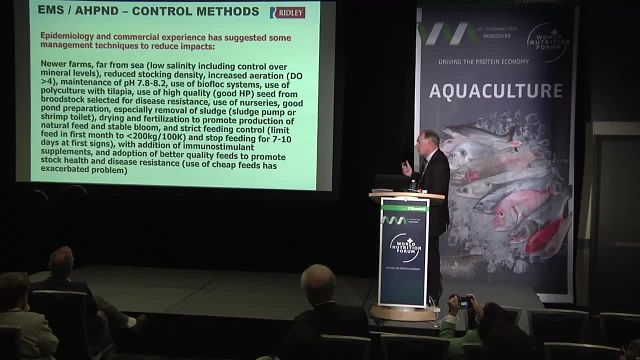 which is basically accumulating all the sludge, and then we can get rid of it out of the pond. Strict feeding control- very important. You have to stop and reduce and stop the feeding as soon as you notice the problem coming. That helps them to recover from it. 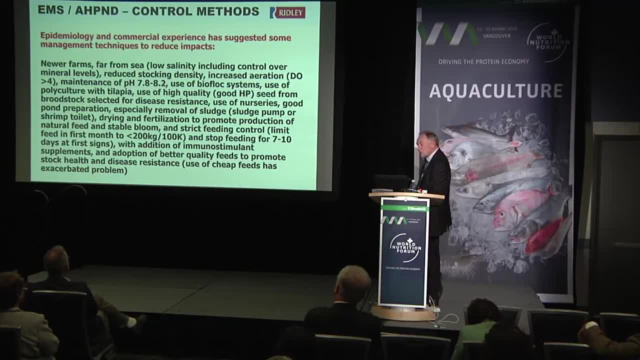 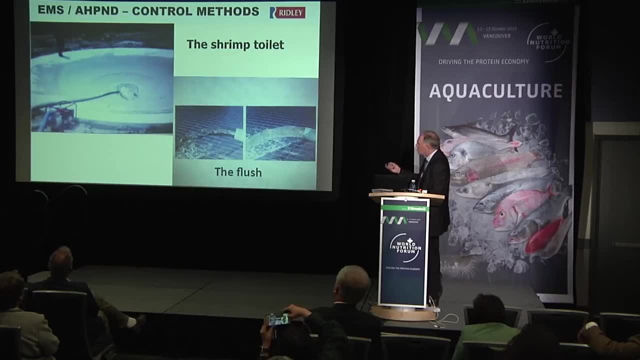 And the use of better quality feeds which promote the stock, health and the disease resistance of the animals. This is a picture of the shrimp toilet and the water that's coming out of it. So when it's black like this, you keep flushing the bottom of the pond. 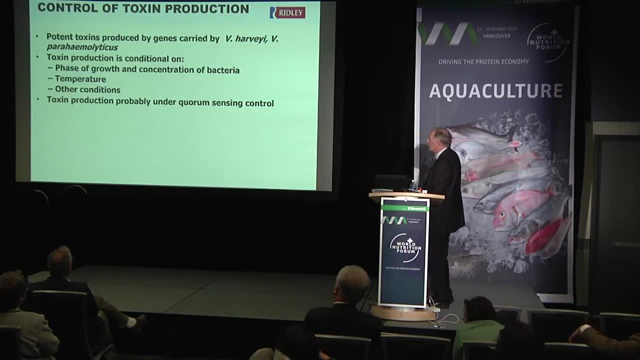 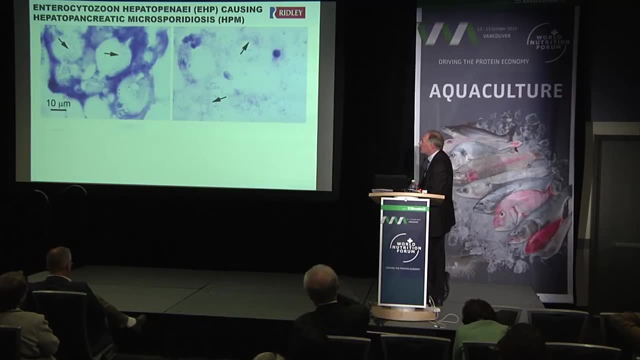 until it turns clear, then you turn it off. I'm not going to go through this one. The other problem that has reared its head recently is this microasperidium parasite, which is a kind of fungi really, And we found that this now occurs. 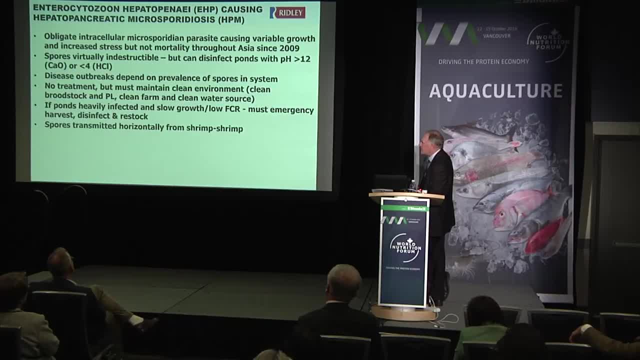 in up to 50% of the ponds. It's very difficult to get rid of it. We just have to maintain the environment as clean as possible. The broodstock are clean and free of it, The PL likewise. We clean the farm and we clean the water. If the ponds become heavily infected, you just have to harvest them and get rid of the animals. There's no other way of surviving with it. Unfortunately, the spores of this microasperidium are transferred directly from shrimp to shrimp, which is quite unusual for microasperidium. Which makes it very difficult. And the shrimp, just they don't die, but they don't grow more than 12 grams, so they've got less value And the cost of culture is higher than the value you get for those shrimp at the end of the day. 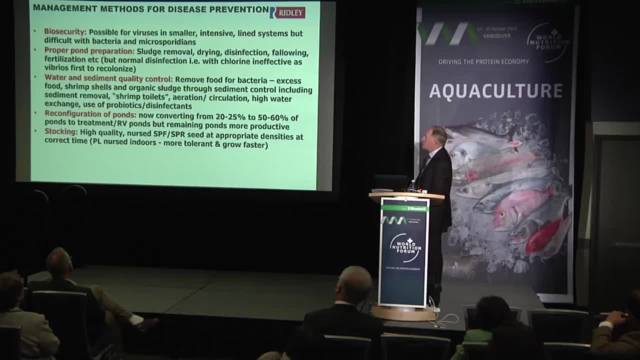 So for management methods, for disease prevention, you've got biosecurity. Very, very difficult with bacteria or with microasperidiums. There's pond preparation, There's sediment and water and sediment quality control. This is really important. Reconfiguration of ponds. 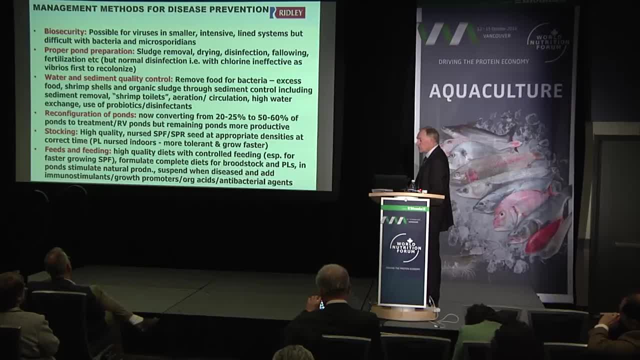 whereby before all of the ponds of your farm, or virtually all of them, were used for production. Now they're converting a lot of those ponds into reservoirs and recirculation and bioremediation- up to 60% of them.